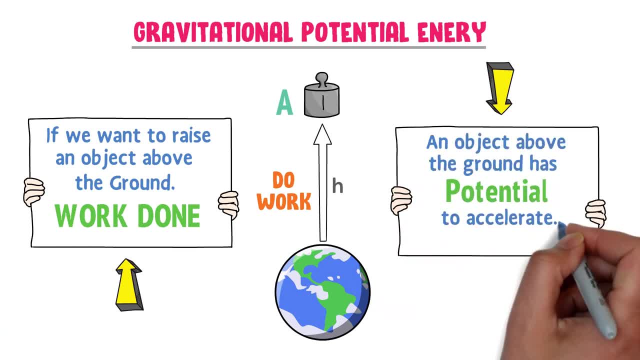 above the ground has potential to accelerate or to fall down towards the ground due to gravitational force. This falling potential of an object due to gravitational force is called gravitational potential energy. Let me repeat it: This falling potential of an object due to gravitational force is called gravitational. 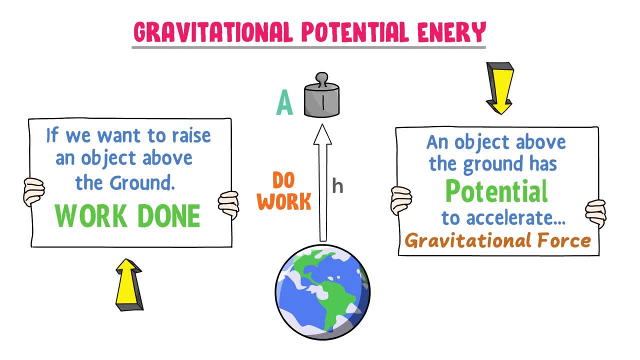 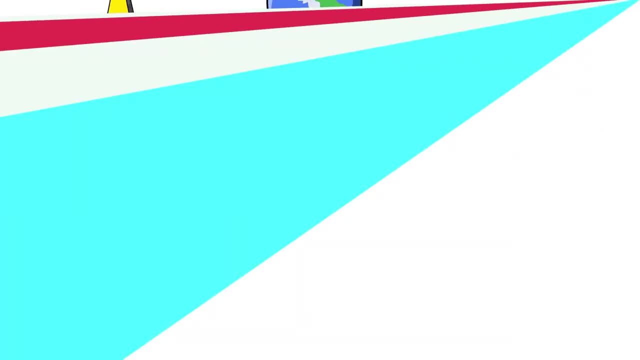 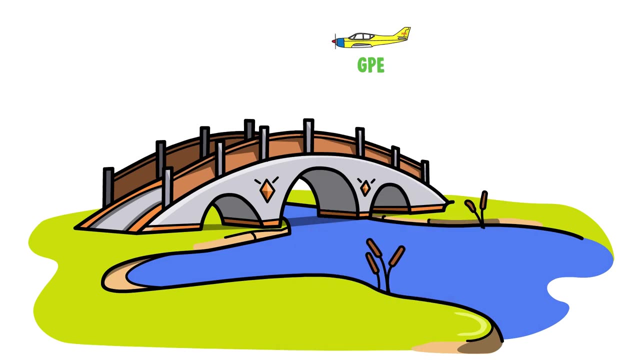 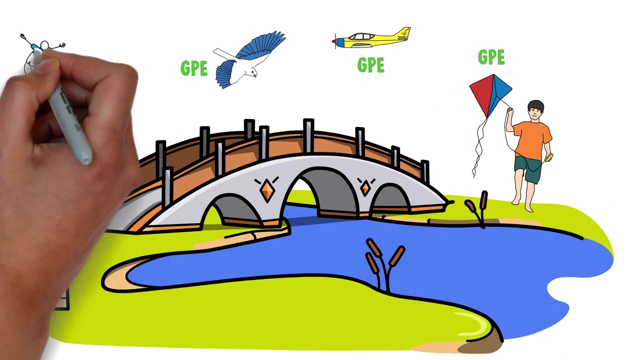 potential energy. Thus we learn that an object, if left up or raised above the ground, possesses gravitational potential energy. For example, the airplane moving above the ground possesses gravitational potential energy, The birds flying above the ground possesses gravitational potential energy, The kite above the ground possesses gravitational potential energy And a man standing 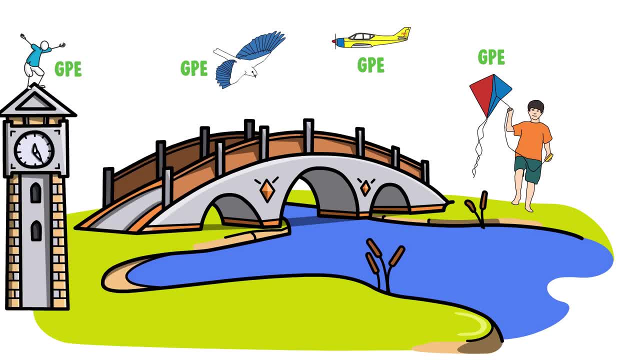 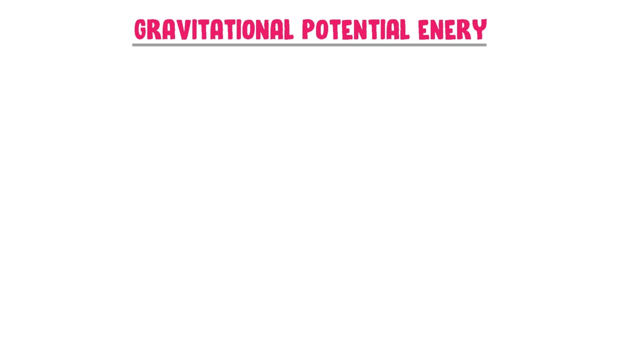 on a tall building possesses gravitational potential energy. Thus, anything above the earth's surface possesses gravitational potential energy. Now let me derive the expression or formula of gravitational potential energy. Well, let's consider that a ball is present on the ground- ground. Let the mass of this ball is m. I exert vertical force f on this ball. As a result, 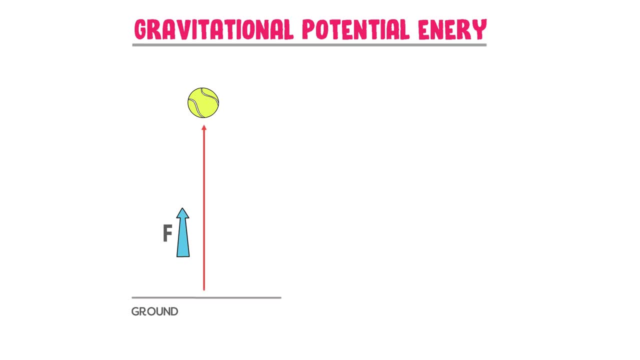 the ball moves in upward direction and gains vertical height h. We know that burden is equal to force and to distance. Here I have done some sort of work on this ball Because I exert force f on the ball and it covered vertical distance h. So burden on the ball is equal to f and to h. 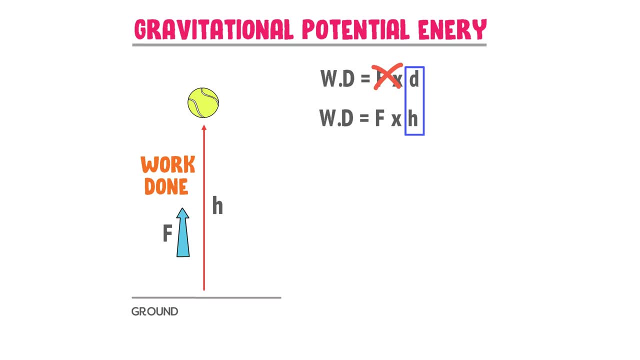 I replace d by h, Because here the ball covers vertical distance h. Let I call this equation number 1.. We know that mass of the ball is m. According to Newton's second law, f is equal to m- a. It means that when I exert force f on the ball of mass m, the ball accelerates in vertical. 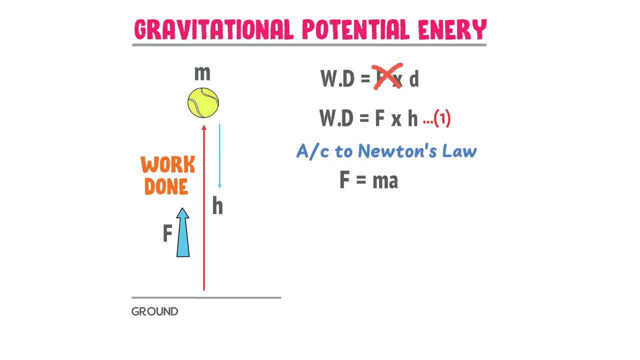 direction. We also know that when this ball falls down, its gravitational acceleration is constant, which is represented by small g. So instead of a I will put g. in this equation I get f is equal to mg. Let I call this equation number 2.. Now I will put equation number 2 and equation 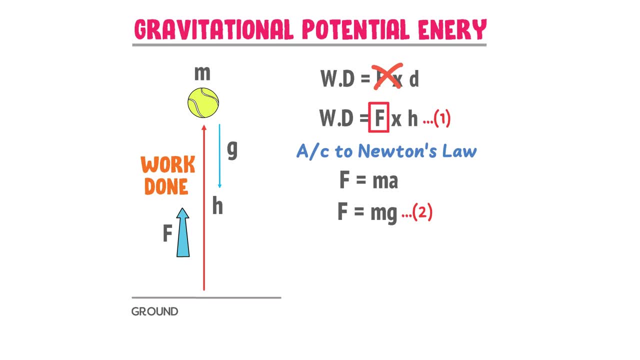 number 1.. Or I will put the value of force in this equation I get: burden is equal to mgh. So our burden stored in this ball is mgh. Let me repeat it: Our burden stored in this ball is mgh. 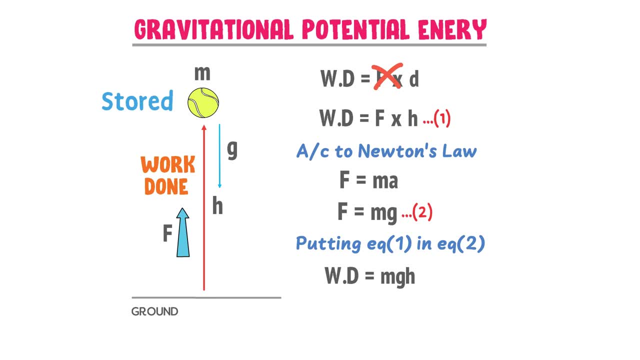 I have said that gravity is equal to mgh. In physics we call this mgh as gravitational potential energy. So the ball above the ground at this point possesses gravitational potential energy. If I ask you why this ball possesses gravitational potential energy at this point, 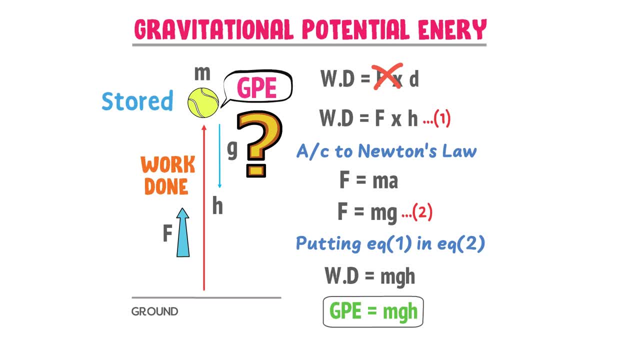 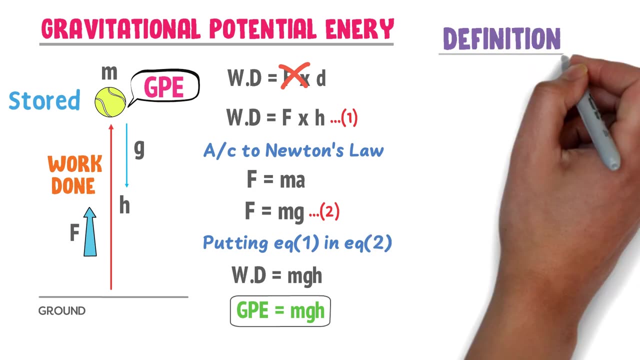 Your answer will be: because I have done some sort of work on this ball and order to lift it up above the ground, and this word uns stored in the ball is gravitational potential energy. Therefore, we define gravitational potential energy as energy stored in an object due to. 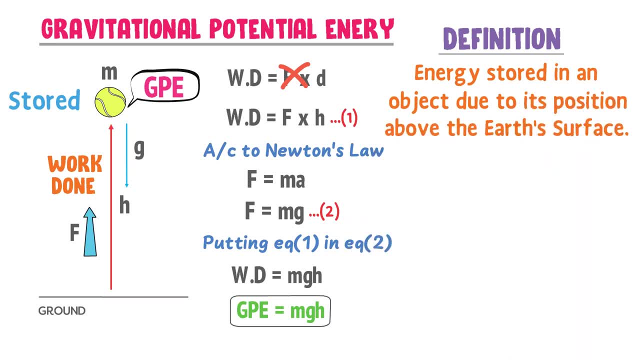 its position above the Earth's surface. Let me repeat it: Energy stored in an object due to its position above the Earth's surface. Note it down that in the formula of gravitational potential energy, m is mass of the ball, which is constant, g is the gravitational acceleration, which is 9.8 m per second squared, and it: 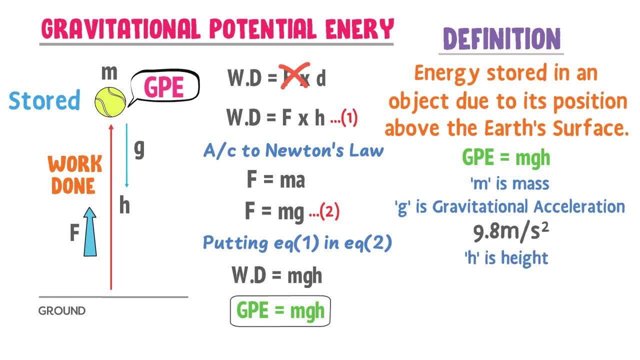 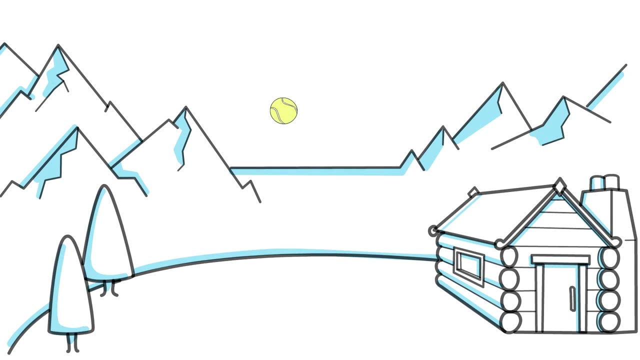 is also constant. h is the vertical height of the ball above the ground. So gravitational potential energy depends only upon the height of an object. Here let me ask you: let consider two balls of same masses above the ground. Let the height of this ball is 10 m and the height of this ball is 20 m.